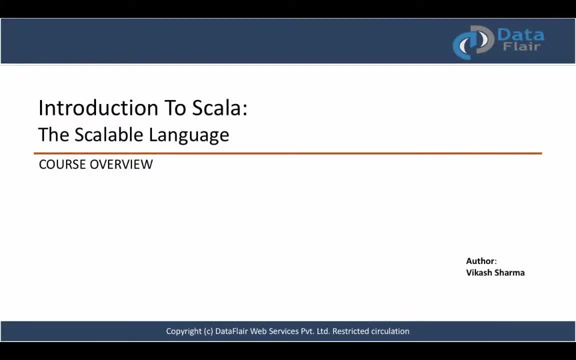 Hi and welcome to this course. I am so excited to bring you this overview course in Scala language. This course might be of real value for a lot of people because, you know right, because of growing industry needs and demands, we need to scale our applications up to get along. and as we are going, 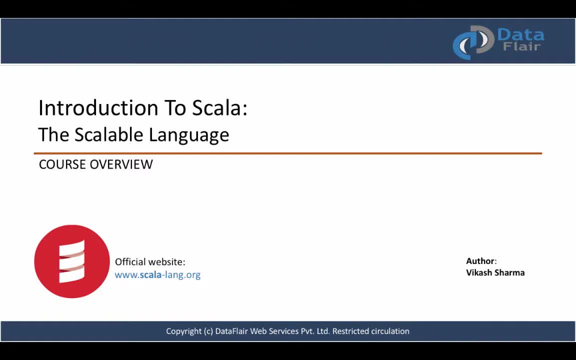 towards achieving scalability in our applications. such languages are here with us to make things easier. It makes it easy to write code more concisely, provides independency for us, the developers, to make our own rules and constructs while writing applications. So, if you're asking me, 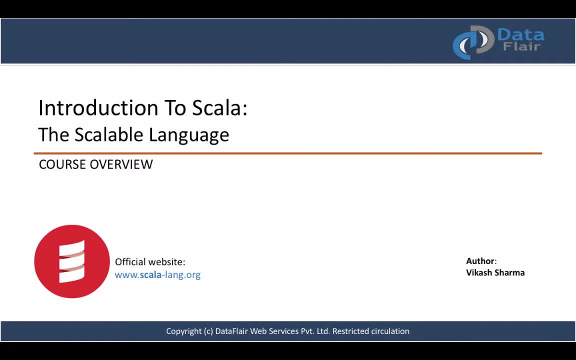 what should you already know to take this course? I'll assure you that there are no prerequisites, but, as you know, it's always an added advantage if you know basics about programming, If you are going to get started with Scala in your very next project. 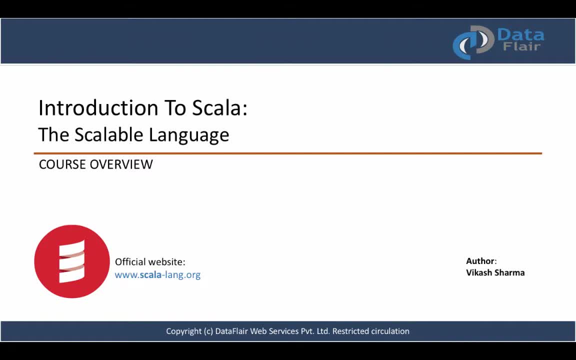 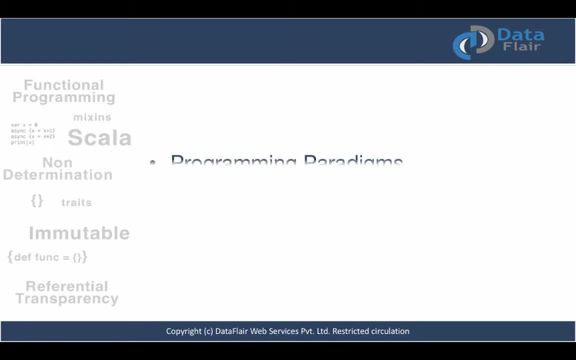 then this course is for you. Next comes: what is our expectations with this course? See, our goal with this course is to make you guys know about what is a programming paradigm and to add a skill set, of course, Scala- to know its history and how it became a popular language. 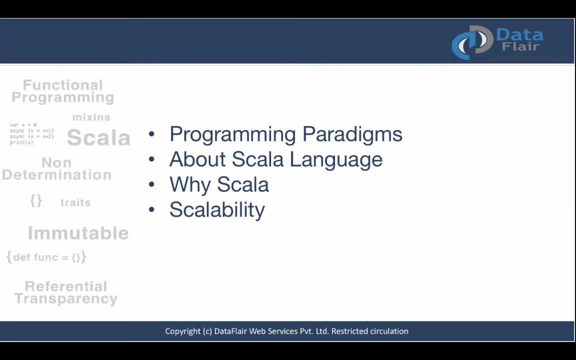 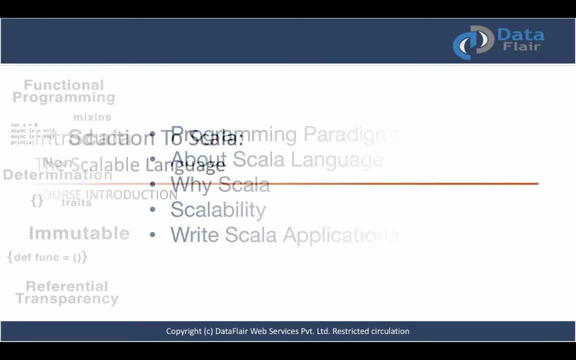 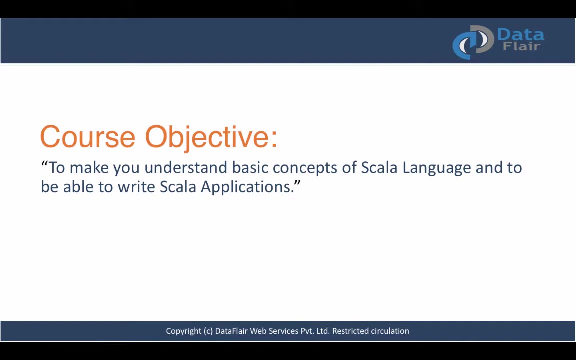 how we can achieve scalability using this language. how it is scalable, I mean to say, and, of course, to write Scala applications, because that's what we are here for. Let's talk about course introduction. Our objective with this course is to make you understand basic concepts of Scala language and to be able to write Scala applications. 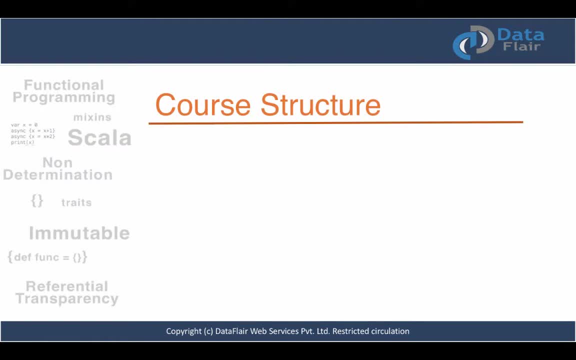 We have divided this course into six modules. With each module we will go further and get comfortable with our understanding of Scala language. First we will start with programming paradigms. We will learn functional programming paradigm. If you haven't heard of this, sit back and relax. we will discuss shortly. 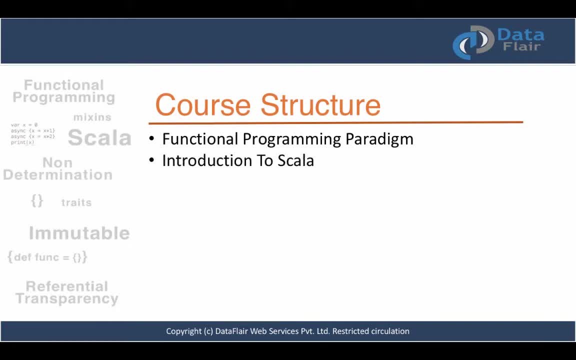 After programming paradigms, we will go on and start our tour of Scala. Then we'll go on and learn about collections. You know Scala has slightly different collections, which primarily supports immutable data structures. Then we'll learn about functional programming: how we can implement functional programming using 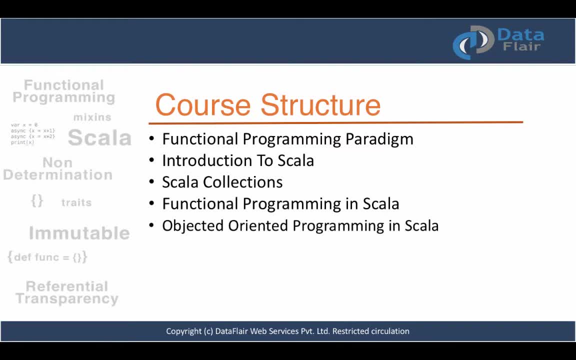 Scala Afterwards, object-oriented programming concepts using Scala, like classes, objects, traits, etc. Because you know, Scala makes sure that you get the best of both worlds. Scala is object-oriented as well as functional, So we will learn about how we can achieve Scala's 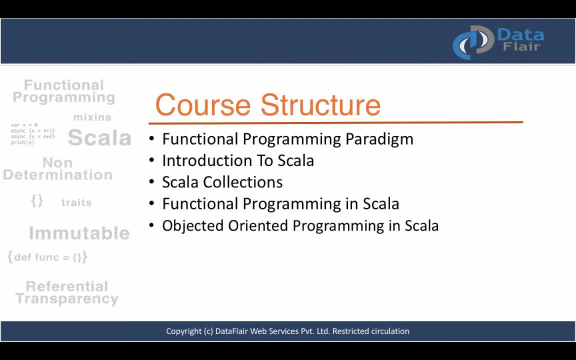 functional and object-oriented capabilities. Then we'll finally dive into some advanced concepts about Scala language, such as the exception handling, pattern matching and how to apply each of these. So put your seatbelts on. we are going to launch our gears and get started. 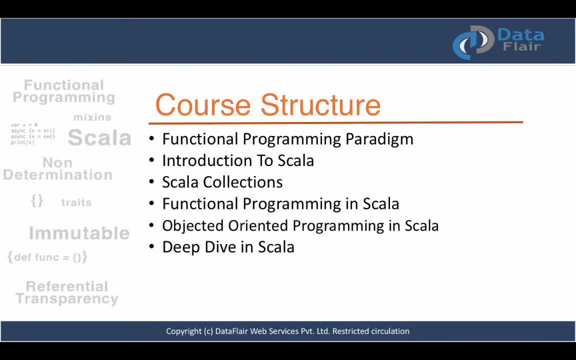 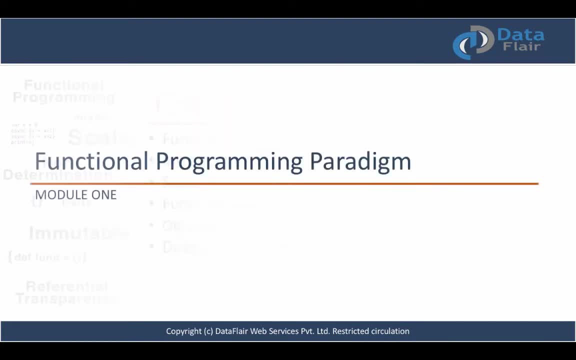 So put your seatbelts on and we're going to launch our gears and get started. all the best in advance, Because you now have done everything you were supposed to do. all know you are done. you know you're gonna scale up your knowledge base now. okay, let's start with. 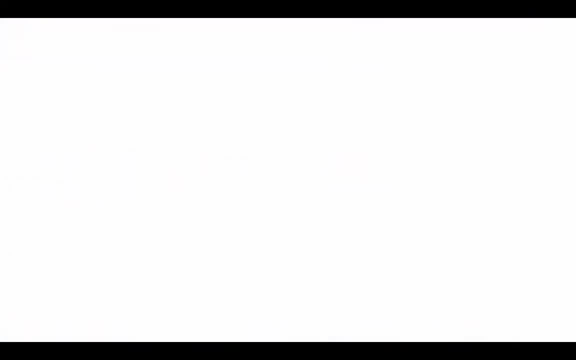 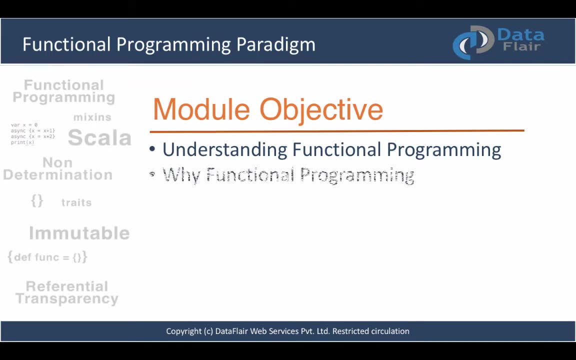 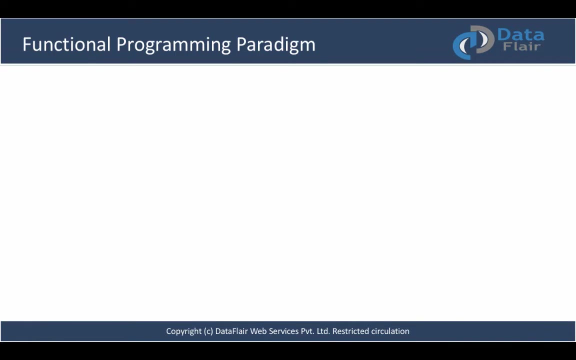 our first module, that is, functional programming. we will be focusing on three major topics for this lecture: understanding functional programming- why is it so important? and able to make presence in modern software architecture. finally, differences between functional and object oriented programming. we will start by discussing what is a paradigm, a simple definition. 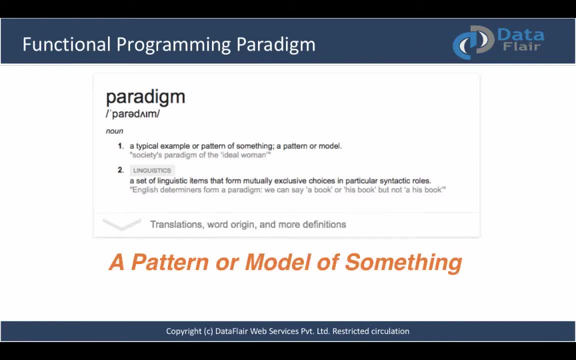 states that a paradigm is a pattern of something, and when we say programming paradigm we mean a pattern of writing programs. the concept of functional programming is old. it is indeed older than you. LISP was the first functional programming language, introduced in late 50s, 1958. what is the main idea of being functional? see, if we sit around the 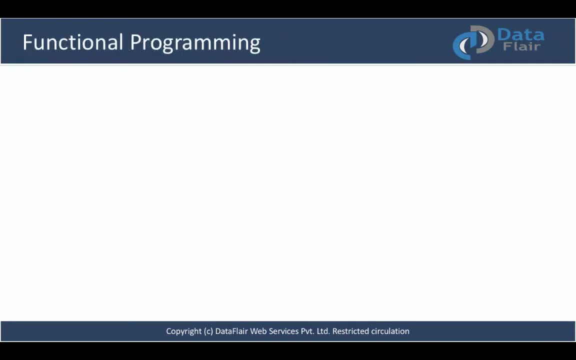 table and discuss about that. we will come up with this argument that functional programming is a pattern of something. and when we say programming functions are first-class citizens, and what do we mean by that? by first-class citizen we mean a function can give meaning to whatever we write. beats an. 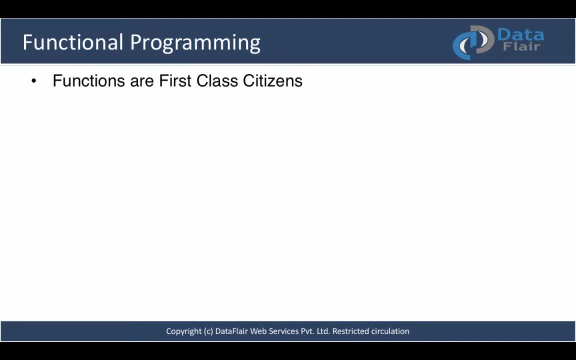 abstraction or some logic to implement. a function can accept another function as a parameter. we can send functions as arguments, we can nest them and be patient. we will take a look at that when we'll do a hands-on layer in this course. second idea is functional programming strongly supports immutability, you know. 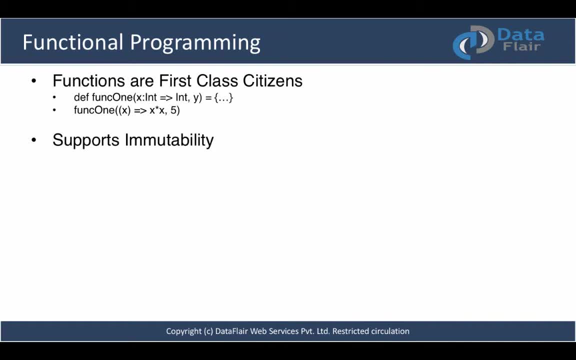 what is it? our friend Wikipedia says an immutable object is an object whose state cannot be modified after it's created. and do remember this property, because later in this course we will relate scalability and immutable objects, and that's why I'll expect you to remember this. so let's repeat this. 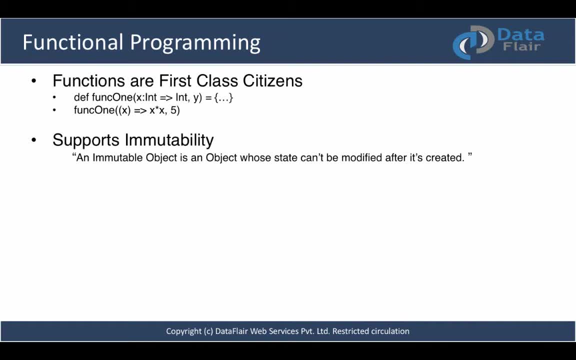 one more time: an immutable object is an object whose state cannot be modified after it's created. great another important concept of the pattern of programming is referential transparency. referential transparency means that functions that you write should expect some arguments and return results after some computation or some logic, without affecting other parts of. 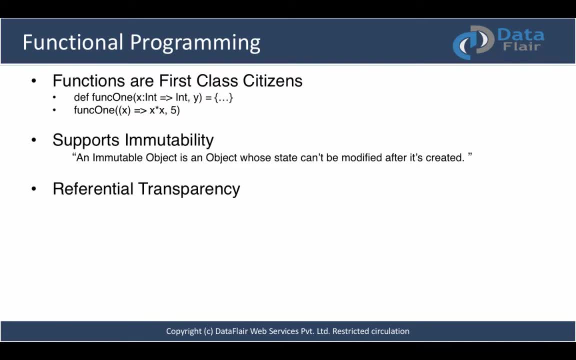 our program, such as state of a variable, etc. let's understand this with this, a simple example. suppose you have this function def, add us together. it's Scala way of writing a function. we use def keyword to define a function, then function name, arguments, list and return type. in our case we are taking 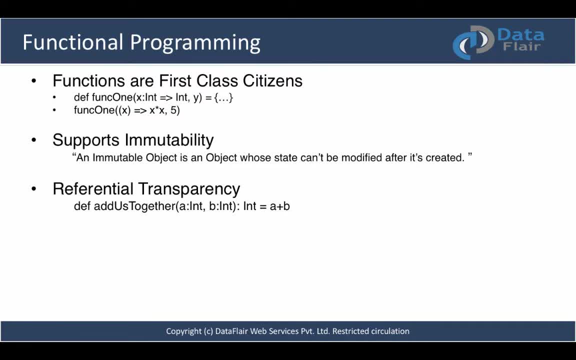 two arguments, a and B. those are of integer type and it's returning an integer. this function is as simple as possible. it performs an add operation and returns back the result. if you look closely, this function does not affect any other parts of the program and supports this major concept of function. 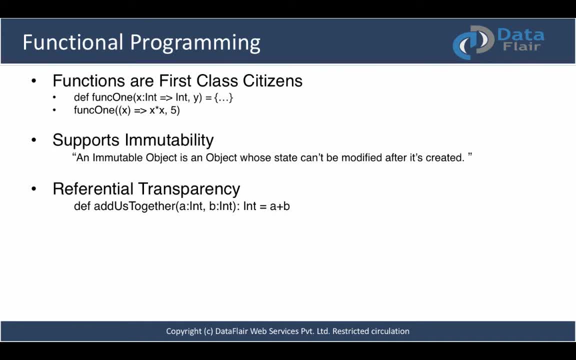 programming called differential transparency. let's define this. referential transparency is a characteristic of a function which states that, for a particular input, an invocation of a referentially transparent function can be replaced by its result without changing the program semantics. let's understand with this example. we will use our add function. 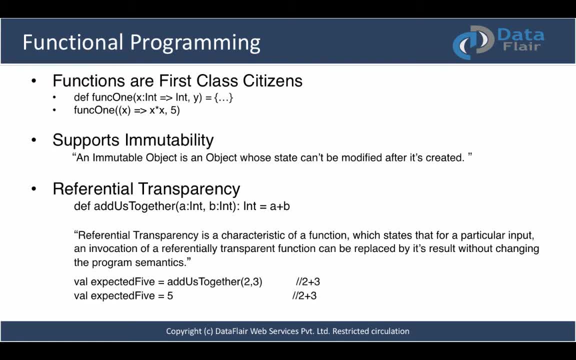 that we defined earlier. we wrote well, expected five, as you can assume that we are going to have five after adding two and three. we are calling this: add us together function. with two and three parameters. it can be written as well. expected five is equal to five without affecting other parts of the. 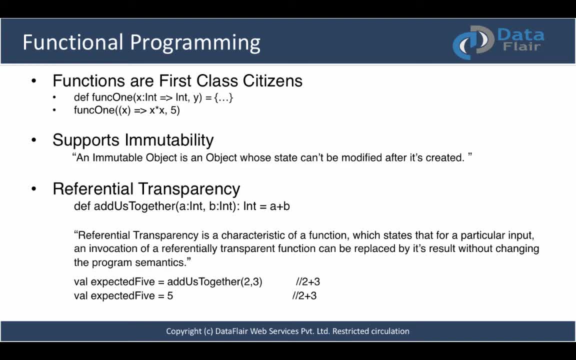 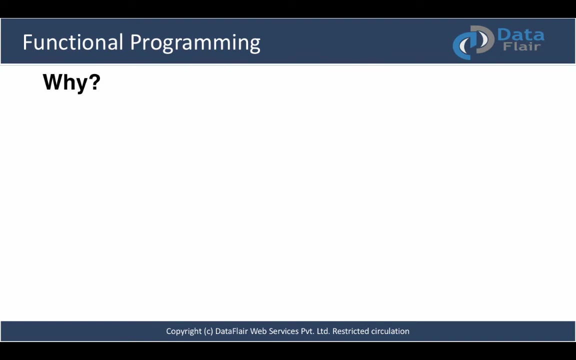 program semantically. so I suppose you understood. and if you support function programming, as I do, you would also support immutable data structures, referentially transparent methods. okay, so let's commit that we are eager and we will look for functional alternatives of imperative constructs. now you may ask me: why functional programming? maybe you just want to start. 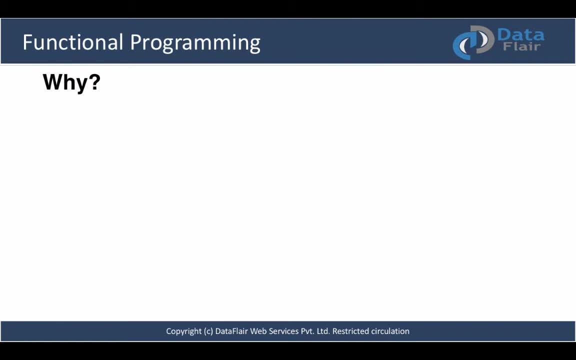 programming and want to know why functional programming- or you would say that I'm so used to and so much into imperative style of programming- why would I choose to go with functional programming? anyway, I'll pause for a moment then my response will be: you know, remember we talked about immutable 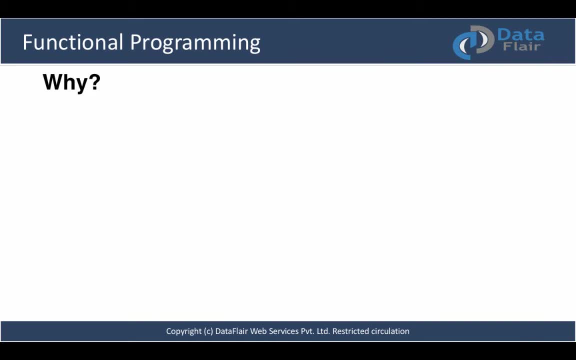 objects. let's relate that to scalability. as a industry is growing up so drastically, small industries grew bigger. their systems are thriving. for scalability, applications used by those industry needs to be flexible with demands. they should be able to scale up or scale down time. scalability is an attribute, meaning to be able to scale up or down in size. 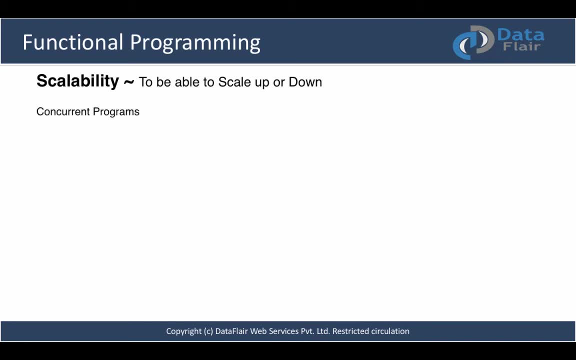 means we need to write content programs that can explicitly execute multiple threads and perform multiple tasks without impacting the overall program semantics. this was hard- managing threads was a cumbersome task and required a lot of hard work- and if you change states of any variable in multiple threaded application, then you are done. this is 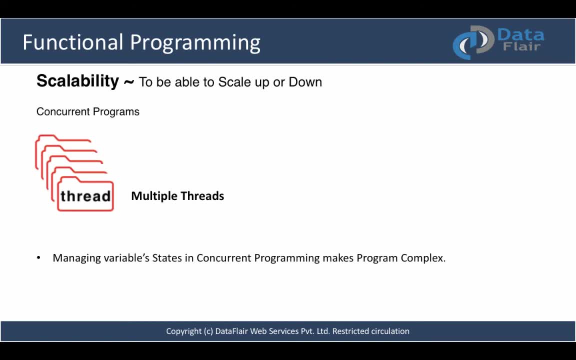 one of the prime reasons of using functional programming. it supports immutability and hence make things easier. immutable objects, once defined, cannot be changed. as we will learn more and more about this way of programming. you see, it's pretty concise. it's pretty and it's concise, and we can achieve more by. 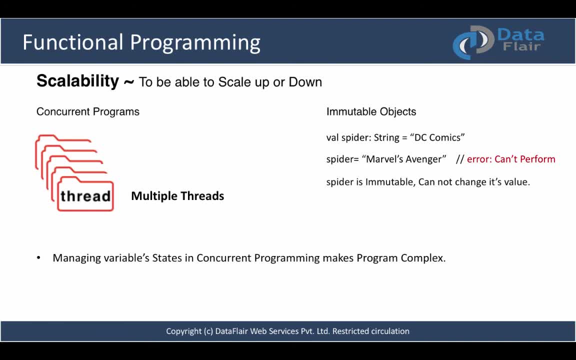 writing less code. and who wants to write more code and get the same results anyway? it cuts down overall time required to produce a scalable and nicely written application. okay, sounds good, isn't it? I suppose you now have some understanding of function programming, and now we'll talk about our 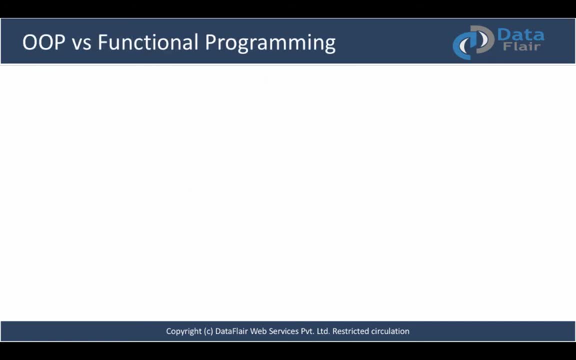 last topic for this lecture, that how it is different from object oriented world. object-oriented programming. provide us a nice way to construct our abstractions. provide us encapsulation in forms of classes. repeat these constructs, get copies of them, call them objects and use them with some logic and get things done. 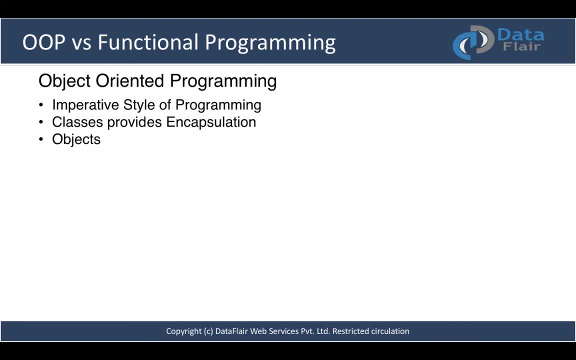 that's how we do it in object-oriented world. but in process of this we play with one sweet little thing called state, which is beautiful to play with if a program is not dealing with more threads. you know you don't want complexity of managing states at all.